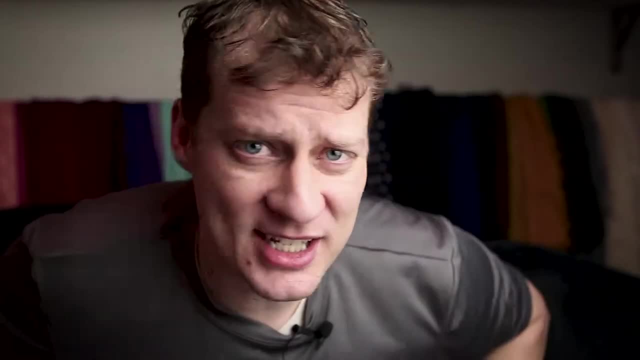 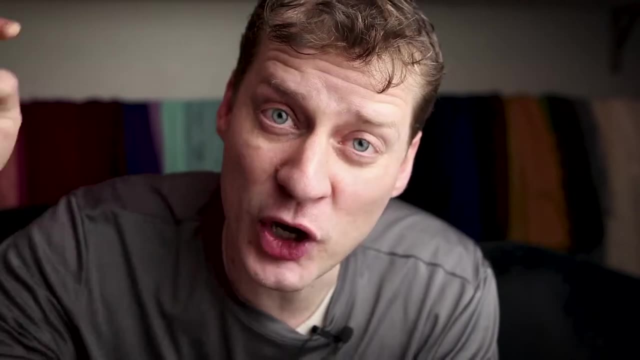 you really can't know the future. The future is always changing. It's always unobtainable And the minute you're just about there it might move and change. Instead, what we do is we take what we currently know about the population and use that to inform our estimate. 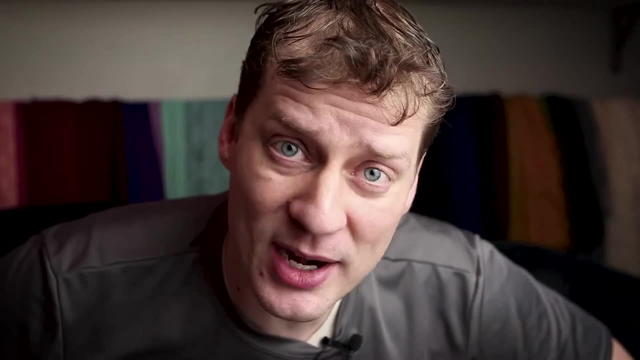 of what the population is. You don't know how many stop lights you're going to hit on the way to work. Well, what's your best guess of what it might be? That's what Bayesians care about, And this belief is what we call a prior. You're not going to get anything from the future. 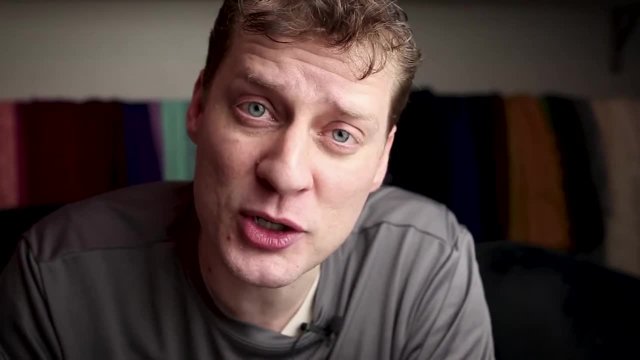 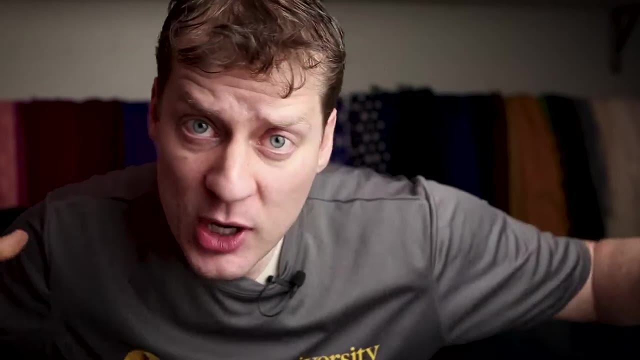 You're going to get nothing from the future. You're going to get nothing from the future meaning it's what we believe prior to performing our actual study. our prior is our best guess of what the population looks like, before we even gather data. so then we go out, we gather some data. so, on your way to work, you actually count the. 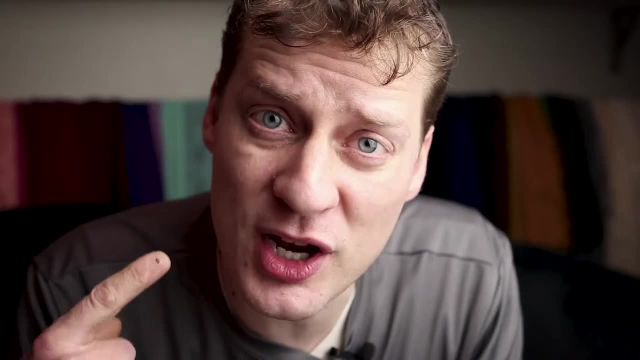 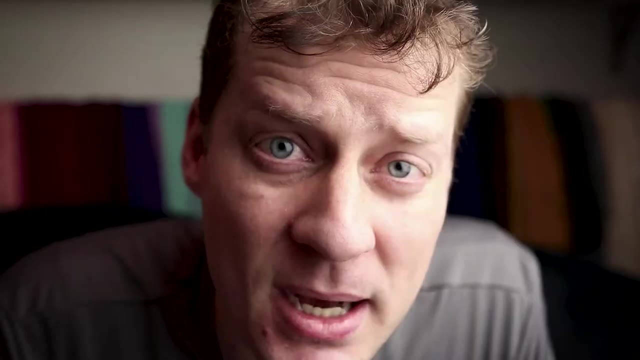 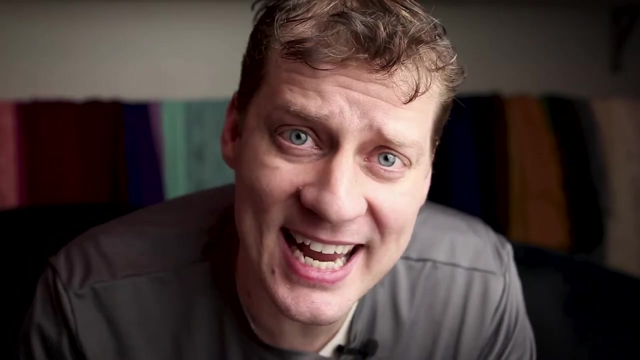 number of stoplights that you hit. and now the data that we collect is going to adjust our beliefs about what the population looks like, and that updated belief now becomes a new prior, but a prior for another study. so, from the Bayesian perspective, estimating the population distribution is an iterative. 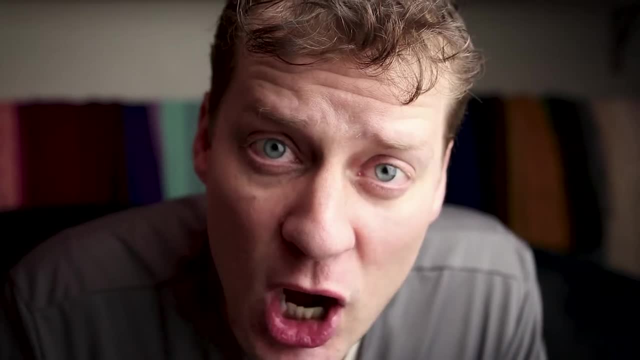 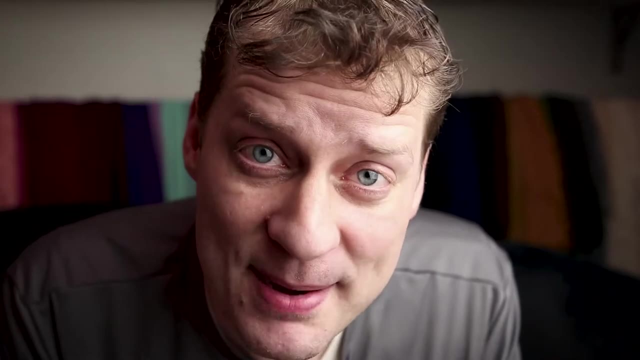 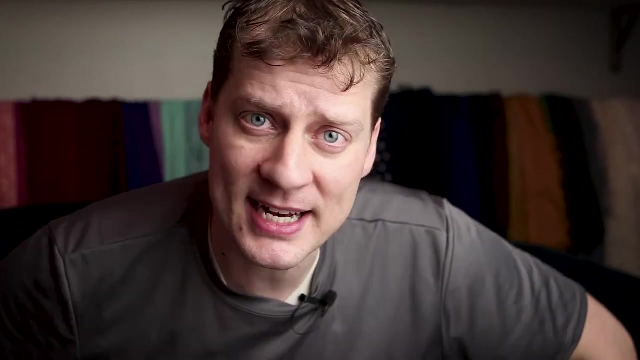 process, one that requires we state our beliefs in concrete terms, collect some data, update our beliefs and repeat and repeat and repeat. over time, our estimate of the population gets better and better. so, for example, maybe my prior belief is that I will hit four stoplights out of ten, but it could be as low as two and as 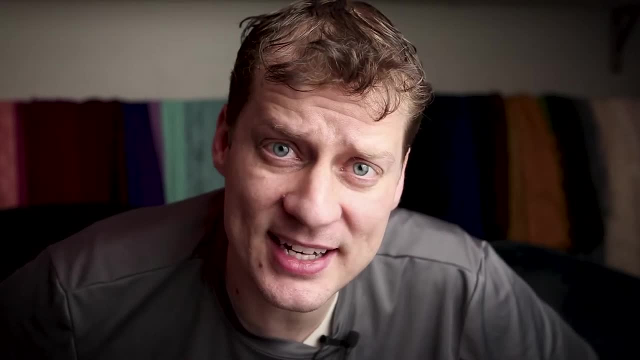 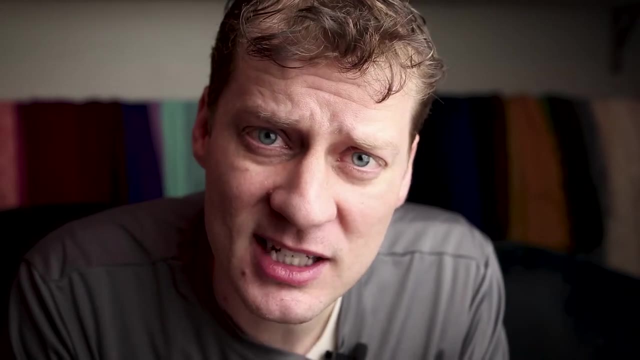 high as six. so maybe I start collecting data and after a week, this is what the distribution looks like. so it looks like we may have been off a little bit, and that's okay, but we're gonna use that to update our beliefs, and so we might say: well, I don't know this. 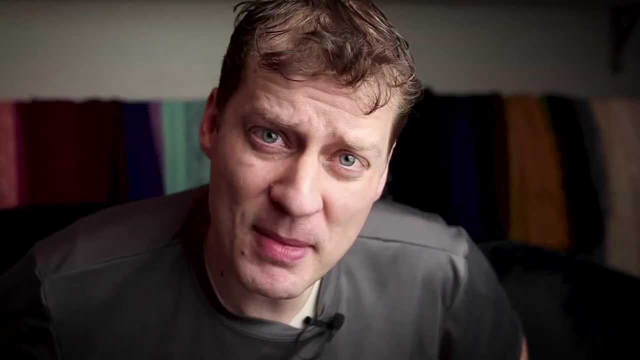 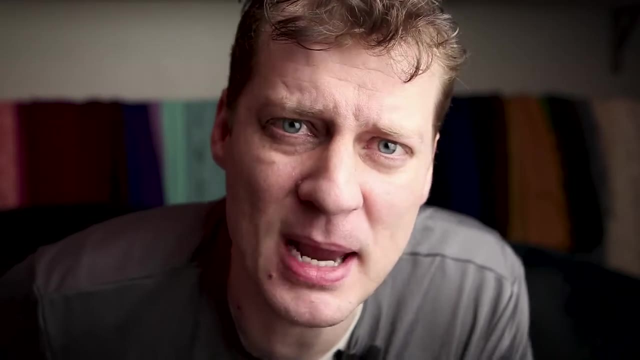 was kind of a good week as far as stoplights go. so now my belief is modified to incorporate that new information. maybe now, instead of saying that I think it's four stoplights, I might say okay, maybe it's three, which is a compromise between what I believe before and what the data are telling me. 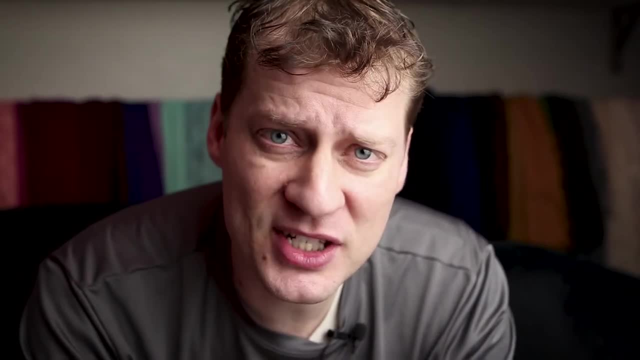 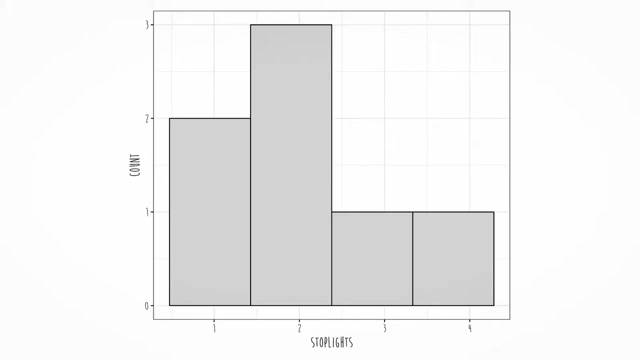 now and, by the way, we call that the posterior, and the posterior is just some aggregation of what we believe before we collect the data with the actual data itself. now, let's say, we do it again for another week and here's what the data look like now. okay, I'm starting to be convinced that maybe my original belief 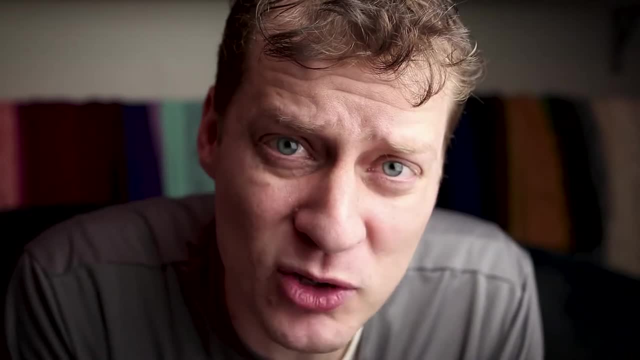 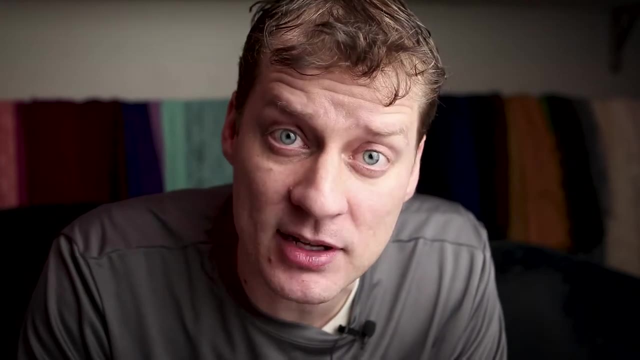 was a little off, so maybe now my initial beliefs are playing very little role in what my estimated population is now. instead, what is playing a much larger role is the actual data that I have collected now suppose I do this for two years. that guy's a nerd. after two years of collecting data, you better believe I. 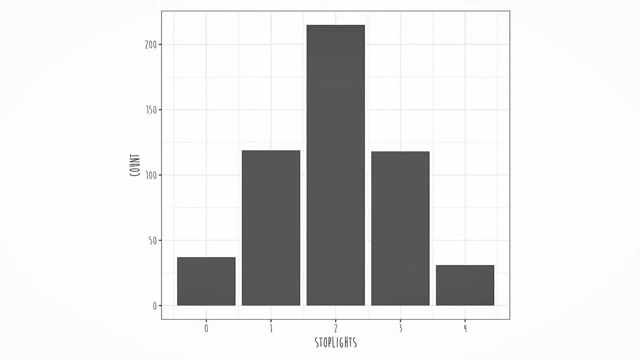 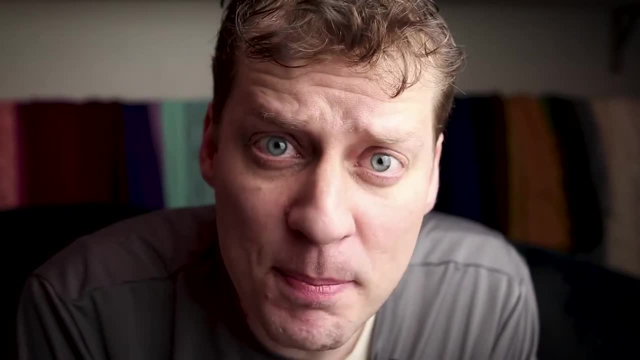 have a dang good idea of what the population looks like, and maybe it looks like this. but now let's say they build a hospital on the way to work. well, snap diggity, my commute just doubled. now the population parameters have changed, and that's just fine with Bayesians- they are. 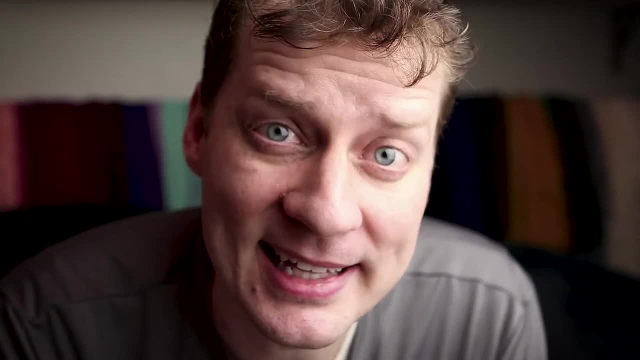 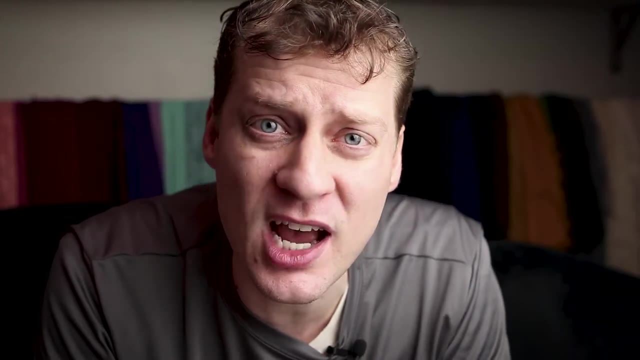 okay. with the population changing, that just means we have to keep collecting data, and that's okay. so let's look at the big picture real quick again. we're trying to estimate something about a population or something that's gonna happen in the future or is otherwise unobtainable, so we collect a sample. 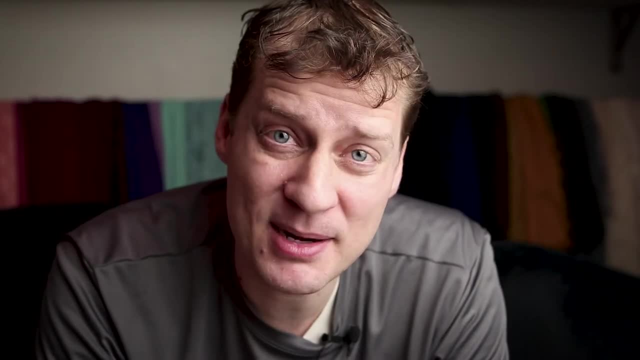 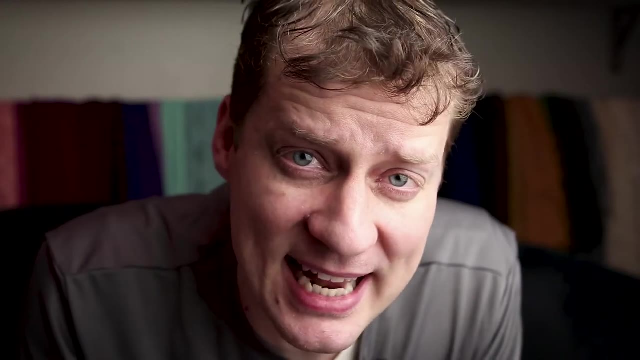 which is gonna be our best guess of what the population looks like. but we know the sample isn't gonna be perfect and so there's gonna be some uncertainty associated with our predictions and our estimates. and we use the sample to estimate the probability density function in some 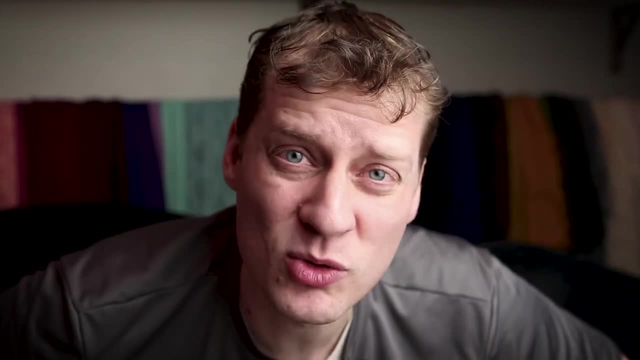 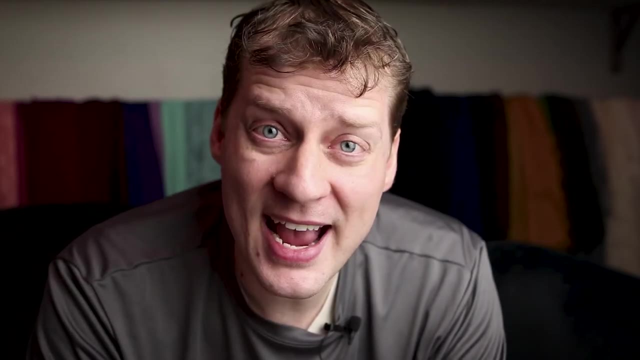 sort of a way. but now, how do we map on what we know about the sample into what we think about the population? the Bayesians would say the way to do that is that you incorporate your prior beliefs or your prior estimate of what the population looks like, and then combine that information with the 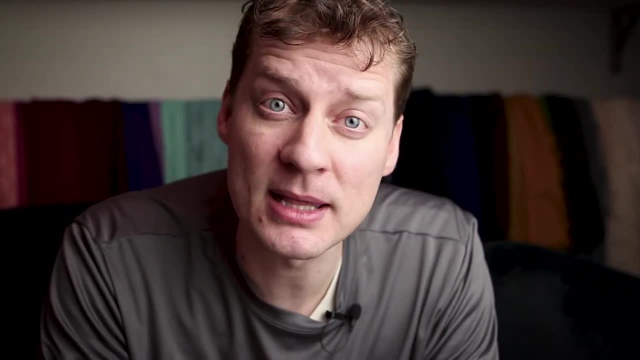 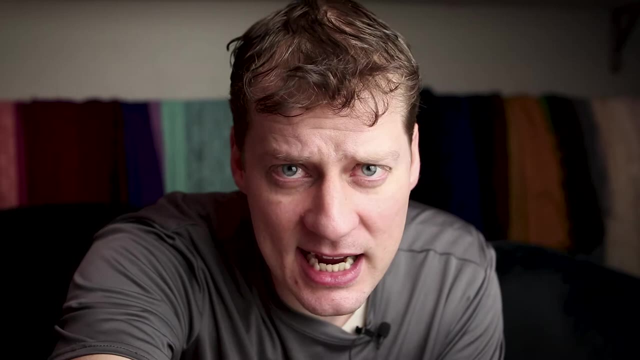 information you collect from the sample and then now we can start making inferences about the population. so that is a very quick and dirty, very diet Bayesian explanation, but that's essentially what it is, and next time I'm gonna be talking about the frequentist or likelihood est perspective, because 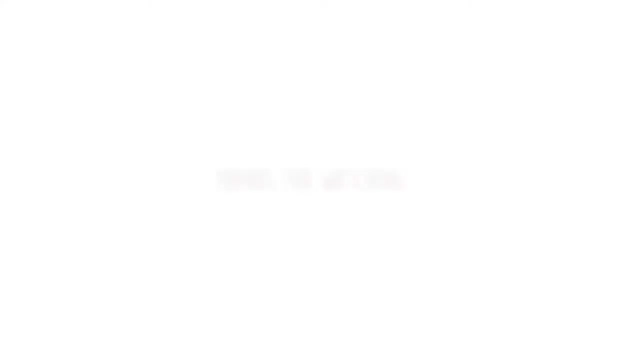 it is very different. I tell you what. until then, peace out. 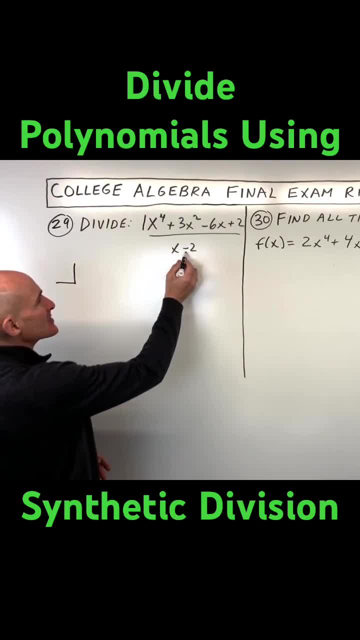 What you want to do is you want to take the opposite, So x minus 2, you want to make this a positive 2.. If this was x plus 2, you'd make this a negative 2.. And then what you do is you take your coefficients, the numbers in front of your variables: 1x to the 4th. 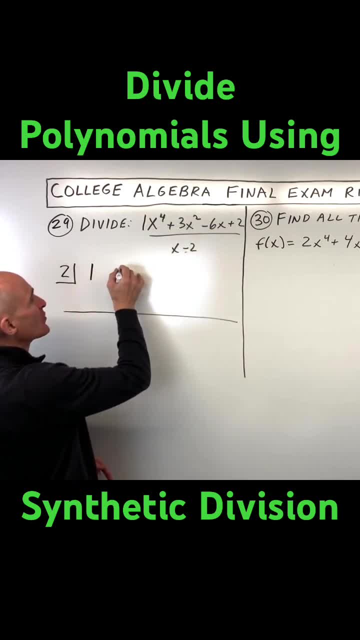 Notice that we skip from x to the 4th, to x squared. We're skipping over x cubed, So we have to put a placeholder: 0x cubed, 3x squared negative, 6x and 2..